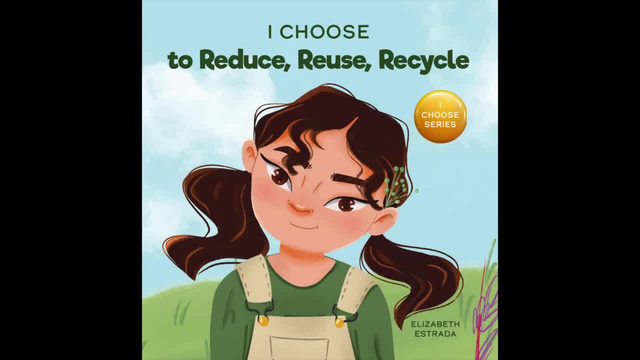 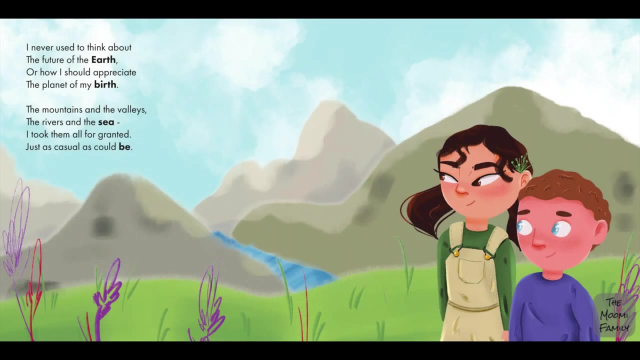 This book is read with permission from Elizabeth Estrada. I choose to reduce, reuse, recycle. by Elizabeth Estrada. I never used to think about the future of the earth or how I should appreciate the planet of my birth, the mountains and the valleys, the rivers and the sea I took. 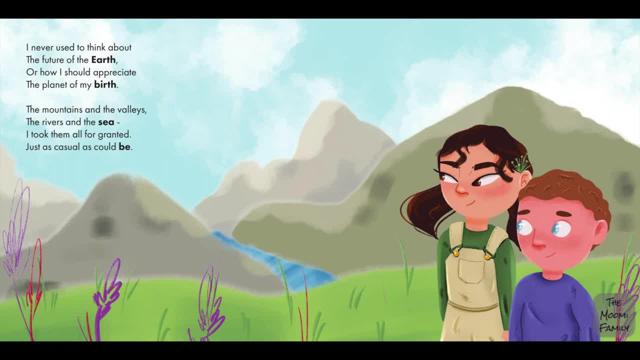 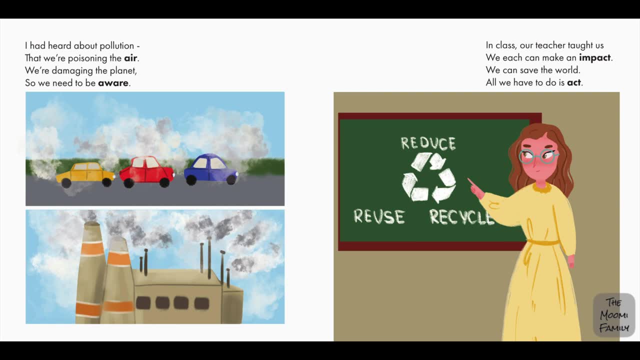 them all for granted, just as casual as could be. I had heard about pollution that were poisoning the air. We're damaging the planet, so we need to be aware. In class, our teacher taught us we each can make an impact. We can save the world. All we have to do is act. 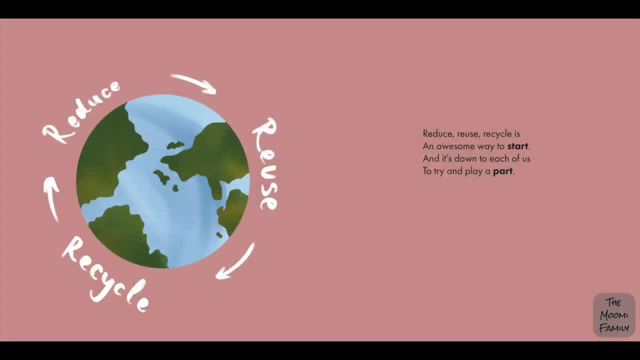 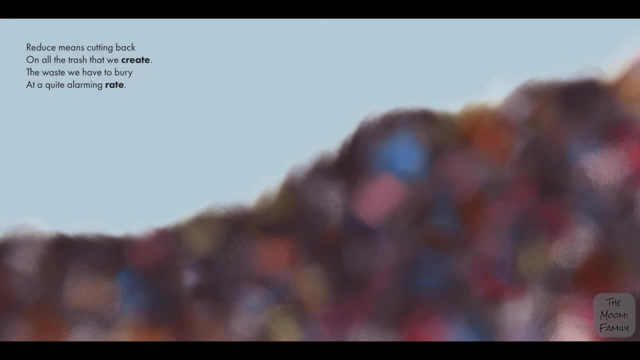 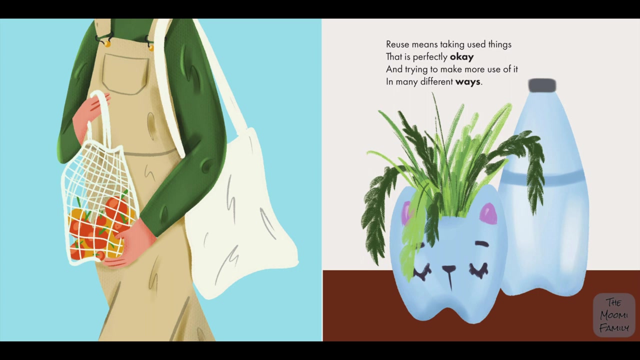 Reduce, reuse, recycle is an awesome way to start, and it's down to each of us to try and play a part. Reduce means cutting back on all the trash that we create, the waste we have to bury at a quite alarming rate. Reuse means taking used things- that is perfectly okay- and trying to make more use of it. 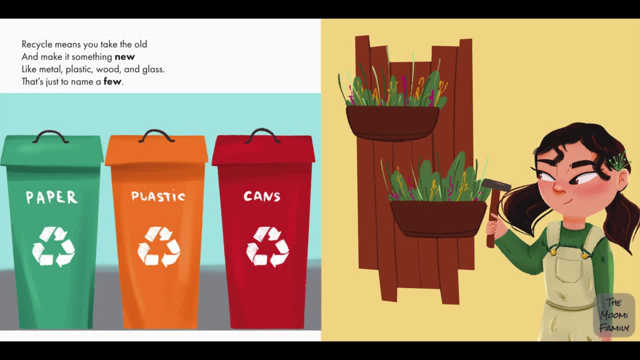 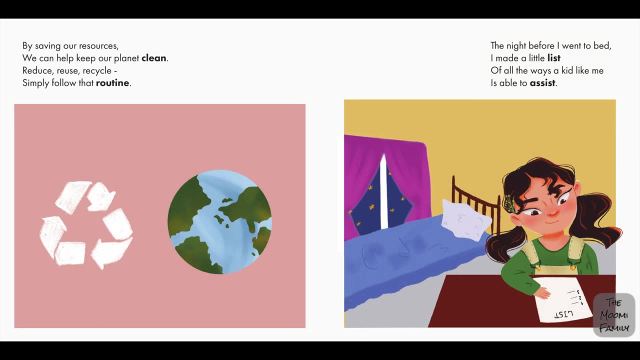 in many different ways. Recycle means you take the old and make it something new, like metal, plastic, wood and glass. That's just to name a few. By saving our resources, we can help keep our planet clean: Reduce, reuse, recycle. 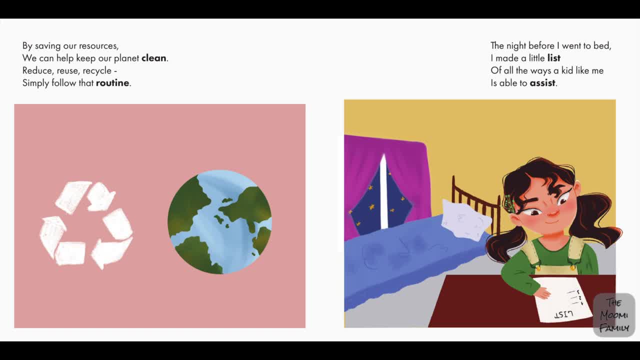 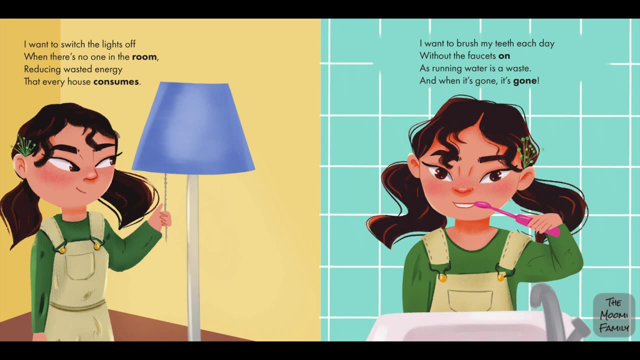 Simply follow that routine. The night before I went to bed, I made a little list of all the ways a kid like me is able to do, able to assist. I want to switch the lights off when there's no one in the room. reducing wasted. 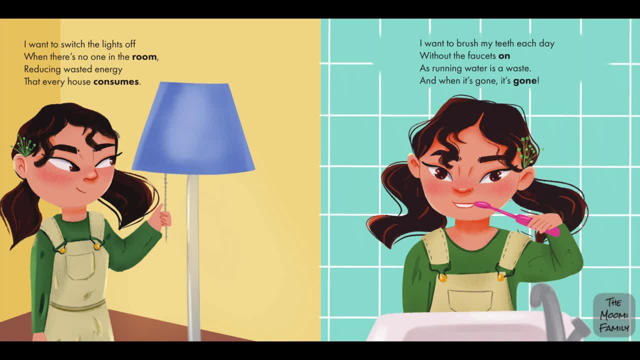 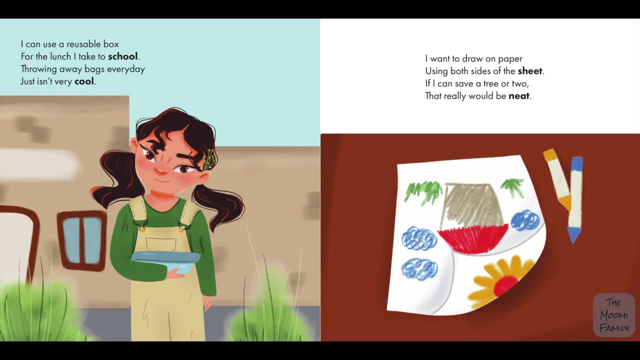 energy that every house consumes. I want to brush my teeth each day without the faucets on, as running water is a waste and when it's gone it's gone. I can use a reusable box for the lunch I take to school. Throwing away bags every day just isn't very cool. I want to draw on paper.